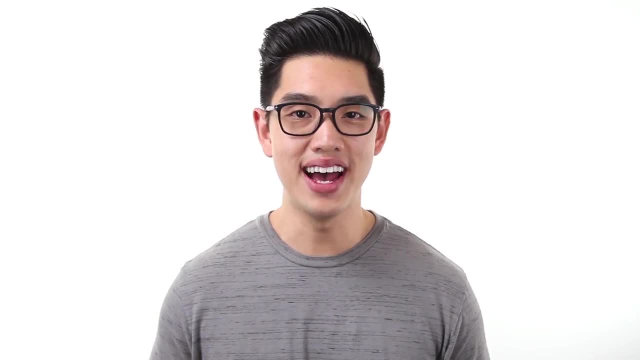 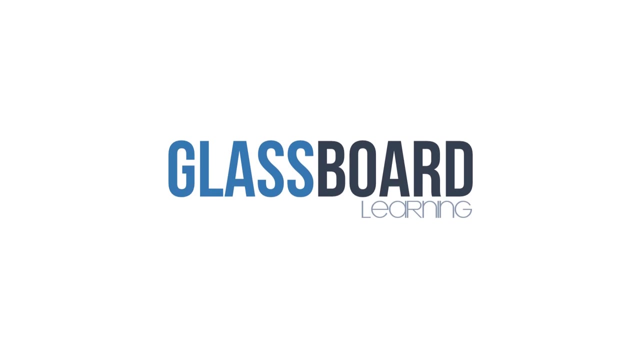 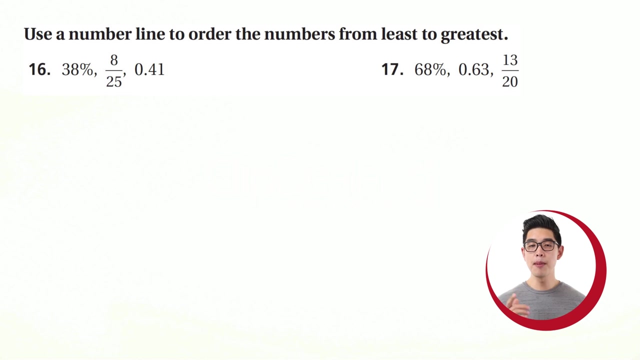 This is Glassboard Learning. I'm Mr Chen. Let's do some math. Here are the problems for today. I want you to pause the video and try them out yourself first. Then press play so you can check your work and your answers with me. 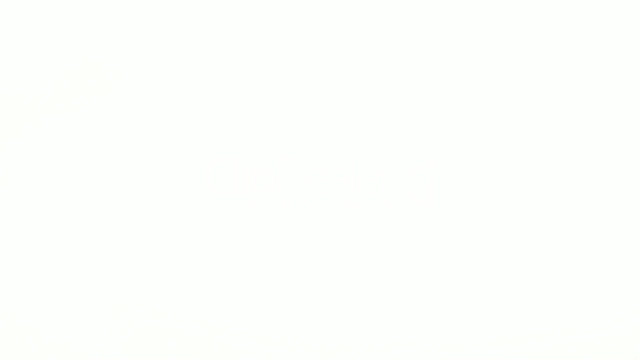 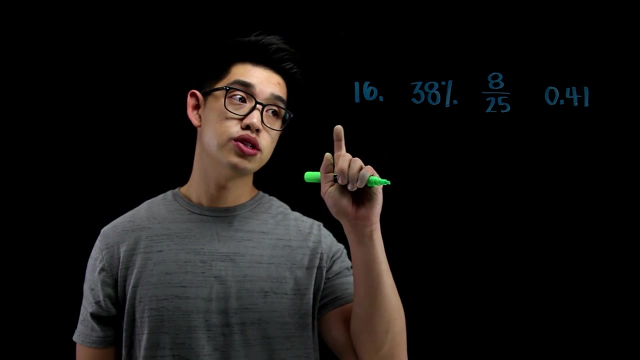 Alright, let's do it For number 16,. I have three numbers. I have 38%, 8 over 25, and 0.401.. My goal is to try to list these three numbers from least to greatest. Hey, there are a lot of different ways that you could do this problem. 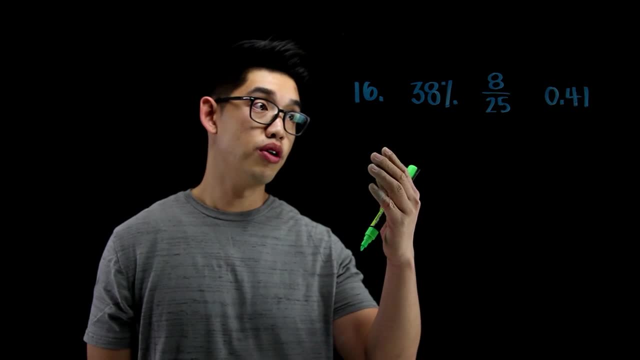 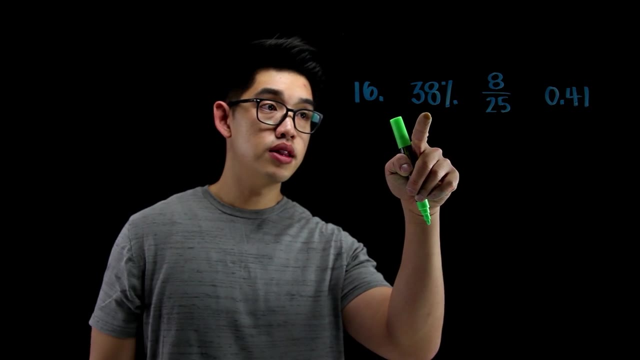 Let me see I could convert them all into fractions or decimals or percents. Let's just make them into decimals, Why not? Let's see I have 38% there. That's the same thing as 0.38.. I want to move it. 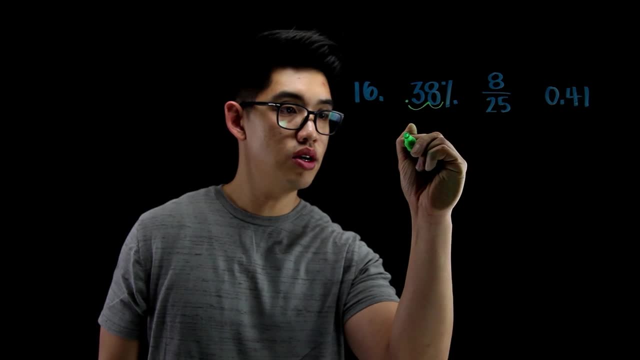 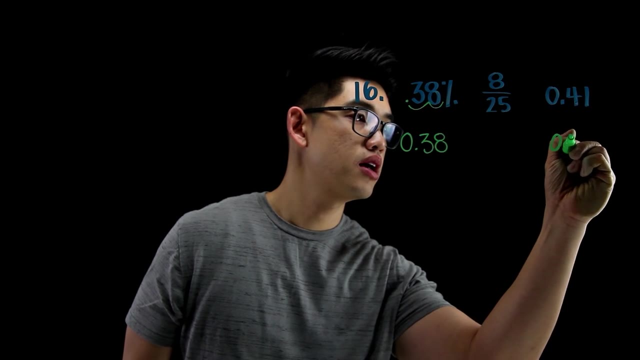 Move the decimal. Move the decimal point to the left two times, That's 0.38.. This one, I'm just going to write 0.41, because that's easy. Really the most challenging one here is this one, but it's not even that hard. 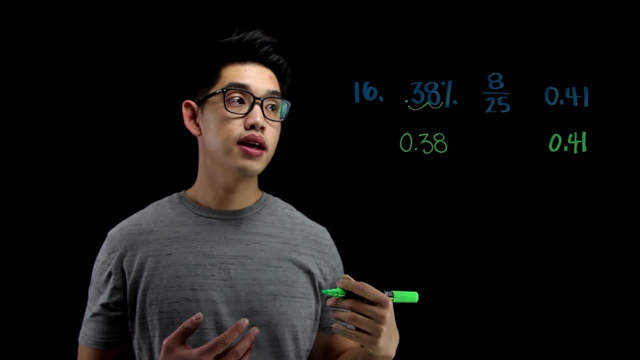 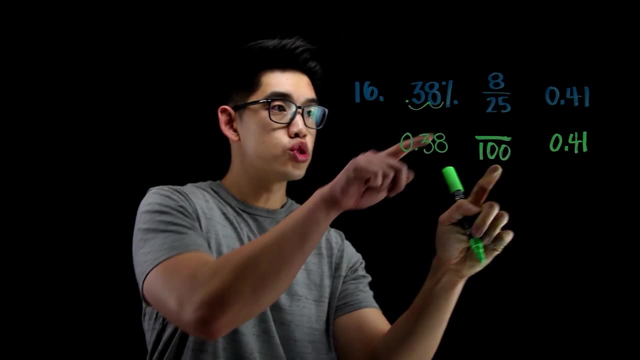 It's 8 over 25.. I want to make it into a fraction out of 100.. I'm going to write 100 here. 25 became 100 because you multiply by 4.. I want to make this equivalent 8 times 4, that's going to be 32.. 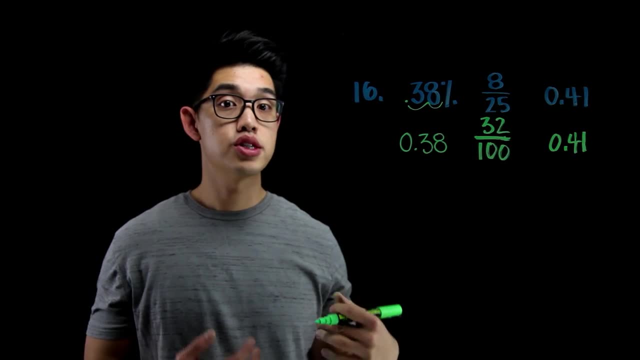 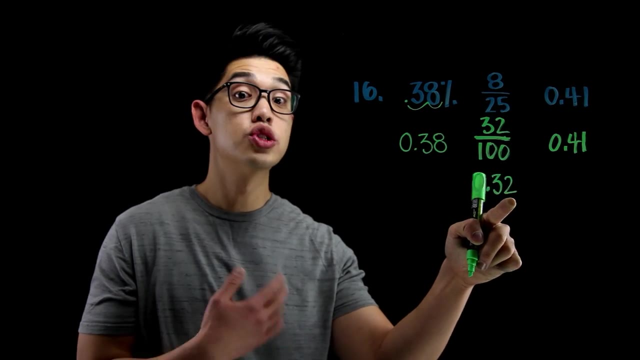 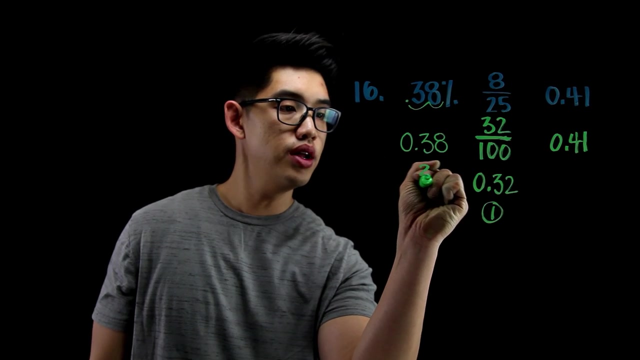 Now 32 over 100, that's the same thing as 32 hundredths. You're going to say 0.32.. That's 32 hundredths. We know that this is the smallest one. The second smallest one is this one: 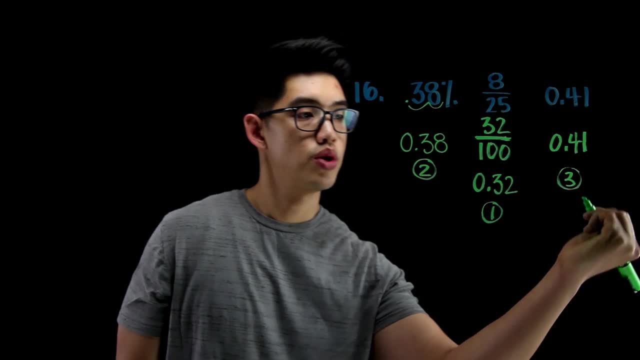 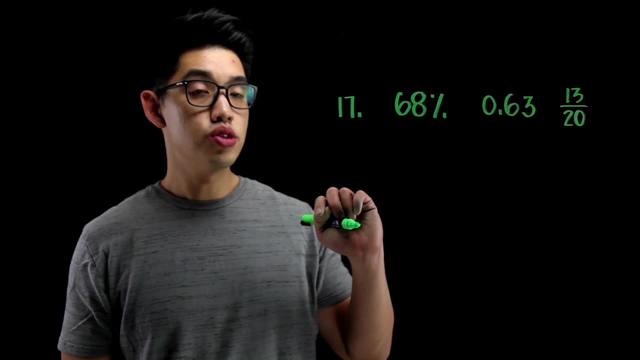 The largest number is this one. I'm going to put a 3 right there. That's your answer For number 17,. I want to do the same thing. I'm going to list this from least to greatest. Let's make all of them into decimals again. 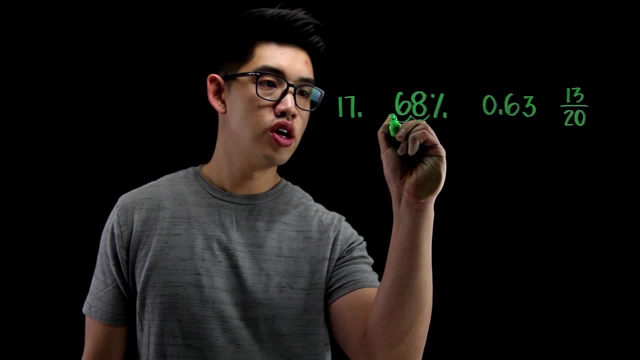 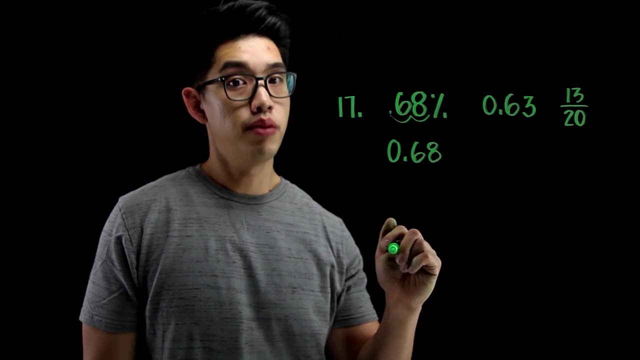 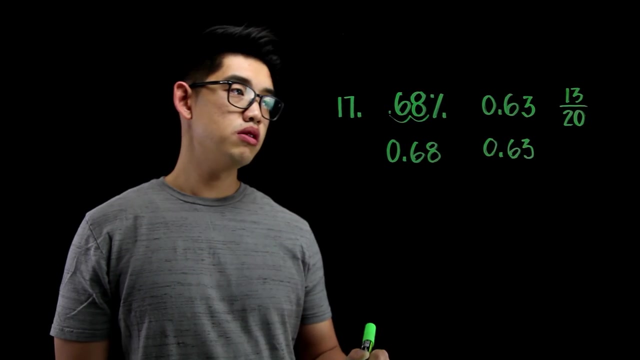 Why not 68 percent? Move the decimal point to the left twice. Put a decimal point there. This is the same thing as 0.68.. 0.63?? Oh yeah, Same thing as 0.63.. Then 13 over 20..